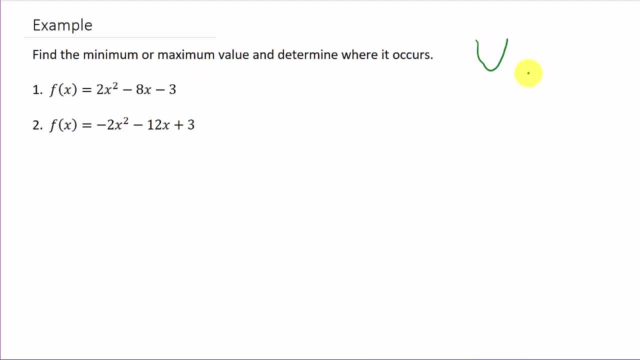 We know it's either going to open up or it's going to open down. Well, how do we know that? Well, you look at the number in front of the squared term. See, in this one it's positive. And since it's positive, we know that the quadratic function opens up. And you can see, here we're going to have a minimum value. Okay, in this one we have a negative in front of the squared term. So we know that's going to open up. 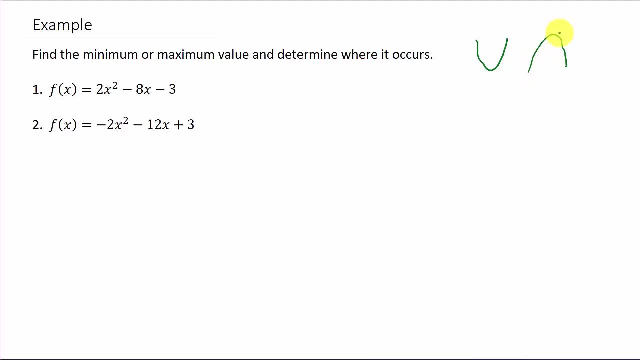 Down And you can see, here we have a maximum value. Okay, so let's look at the first problem. Well, we know it's a parabola that opens up, So we know we're going to have a minimum value, And this value here is called the vertex. Okay, that point is. So what we need to do is find the vertex. Well, if you remember, the vertex of a quadratic function is minus. 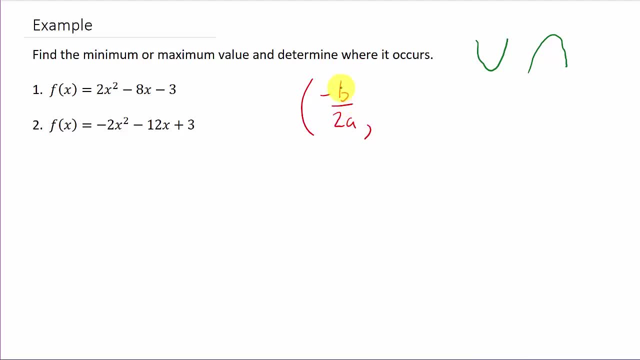 b Over to a. This is the x coordinate of the vertex. And then the y coordinate of the vertex is f of minus b over to a. Okay, this is just the y coordinate. This is the x coordinate. This is the y coordinate. Now, this, this y coordinate. Look, all this means is take this x value and plug it in for x, and that gives you the y value. Okay, So. 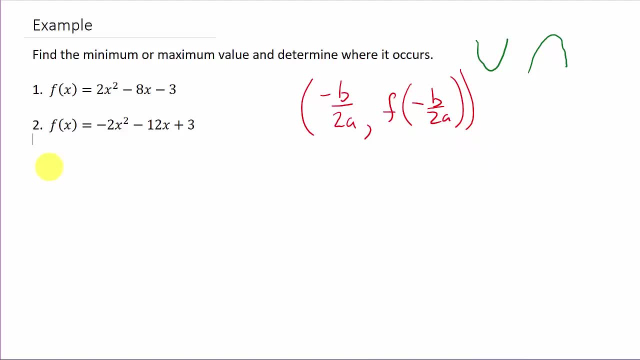 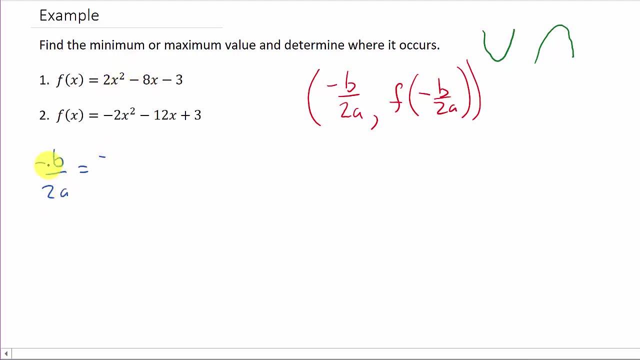 let's go ahead and find it. So let's find. let's find minus b over to a in this one. So that's going to be minus, And then we've got negative. eight is b. Remember the quadratic function. it's in this form: f of x is ax squared plus bx plus c. A is the number in front of x squared, B is the number in front of x and c is your constant. 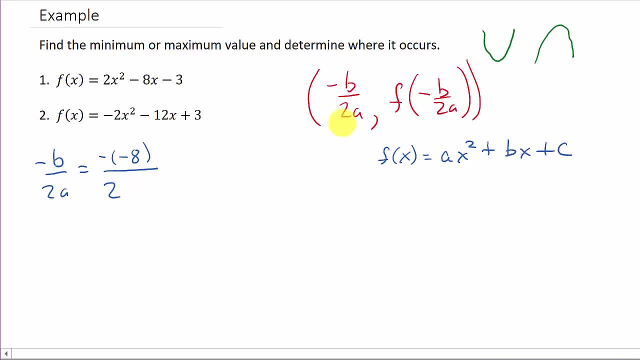 Okay, And that's over two times two times a, And a is two, And so we have eight over four, And so we get, and so we get. the x coordinate of our vertex is two, Okay, So let's go ahead and put that over here. So that's two, And now let's find the y coordinate. So all we do to find the y coordinate is to find the y coordinate. 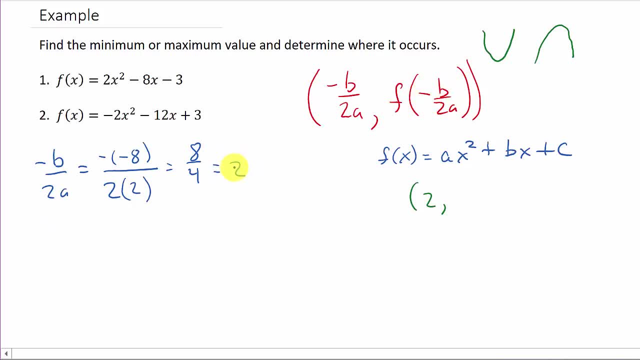 Okay, So all we do to find the y coordinate is to find the y coordinate coordinate is we take this value here, our x value, and we evaluate the function at our x value. so that's 2 times 2 squared minus 8, times 2 minus 3, and so that's 2 times 4 minus 16 minus 3, and so 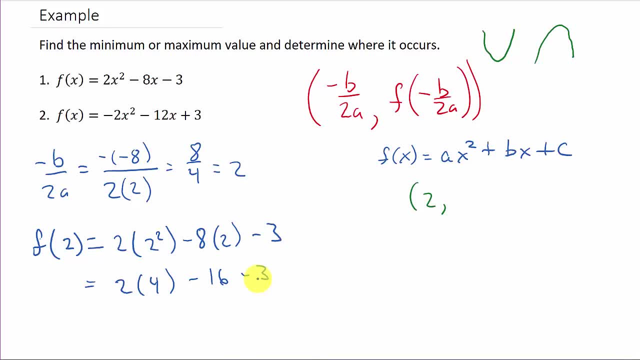 that is going to give us 8 minus 16 minus 3, that is going to give us negative 11, and so the y coordinate is negative 11. so this value, since the parabola opens up, it is a minimum. okay, now let me say this: some books they they may ask for the coordinates. 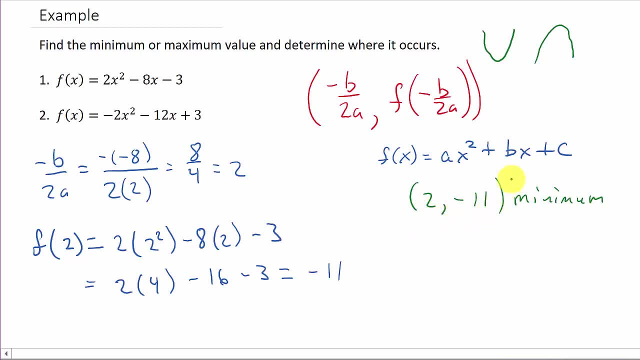 of the minimum, of the minimum or maximum value. if that's the case, this is what you would give them and some books. they'll ask to find the minimum or maximum value, and what they'll want as their answer is: they'll just want the negative 11 is a minimum. they just want the y, the y coordinate. 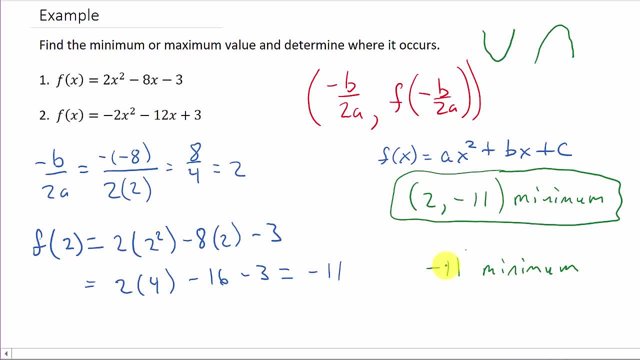 okay, so you know, look at the examples in your book or look in the back and see how they want the answer written. okay, so now let's look at the second problem. let me erase this and you know, if you like the video, give it a like and share, and check out my other videos. 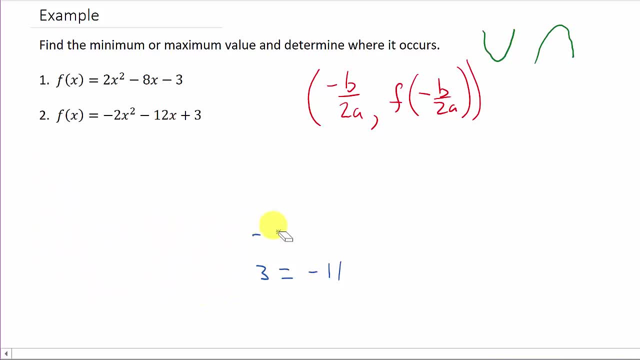 and subscribe if you like them. alright, so now let's. let's look at number two. so we got to find minus B over 2a, So that's going to be negative b and b is negative 12, over 2 times a and a is negative 2..